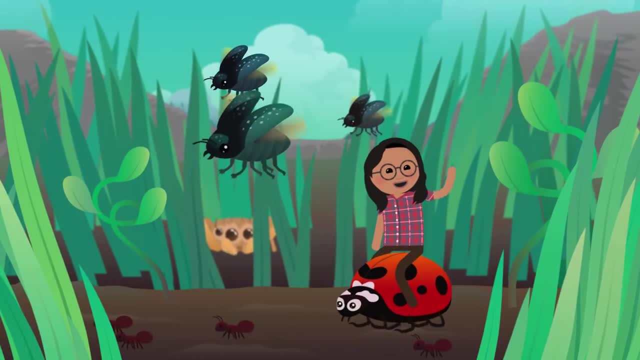 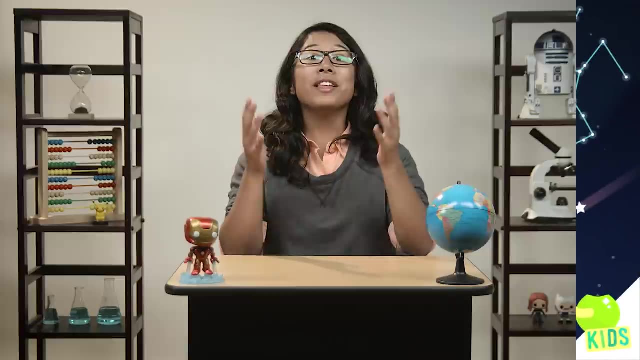 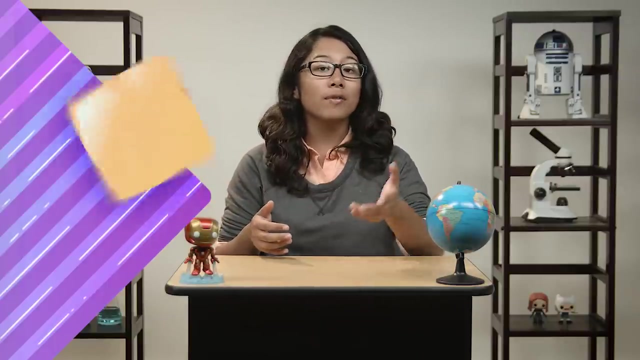 We've spent the last few episodes talking about the effects of the atmosphere on the geosphere and the hydrosphere on the biosphere, as well as solving some pretty big engineering problems. So how about we take a break from Earth this time and talk about space Now? 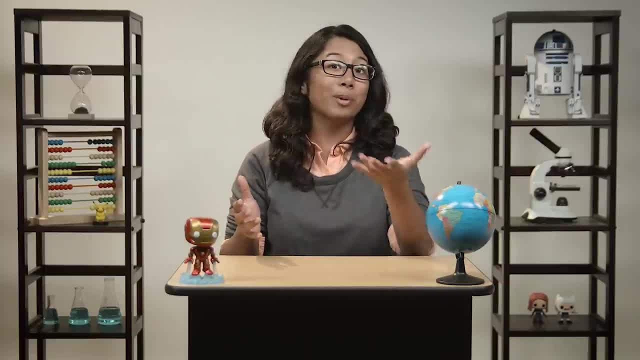 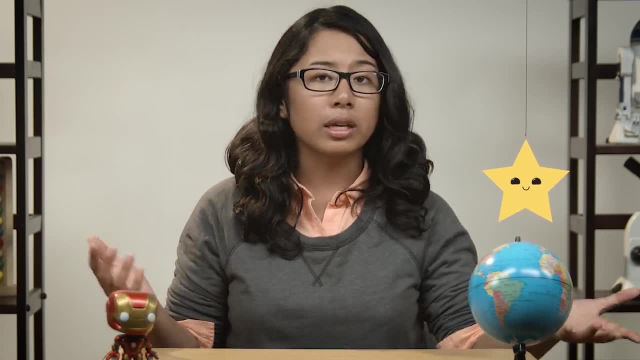 you might be thinking, but we've already learned about stars. Well, you're right, or at least you've been paying attention. But we learned about individual stars, basically how they do what they do as solo acts out there in the universe. But what happens when a bunch? 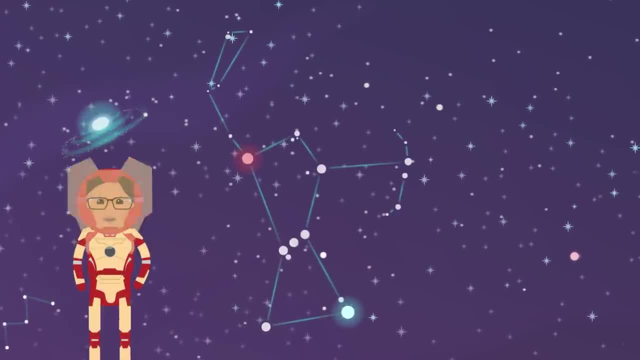 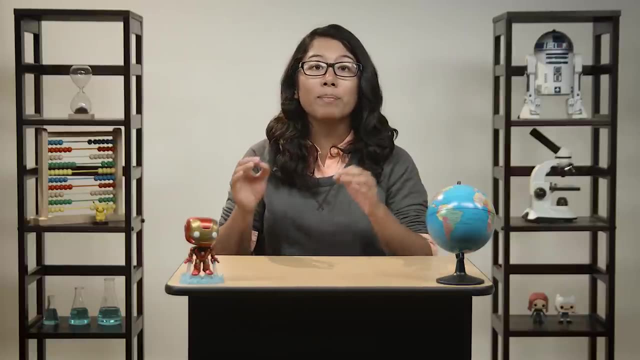 of stars band together to form a supergroup, sort of like the Avengers of the night sky. Well then, they're called a constellation. Today, we'll talk about these groups of stars and why they're so important to astronomers, besides being just plain cool or hot you. 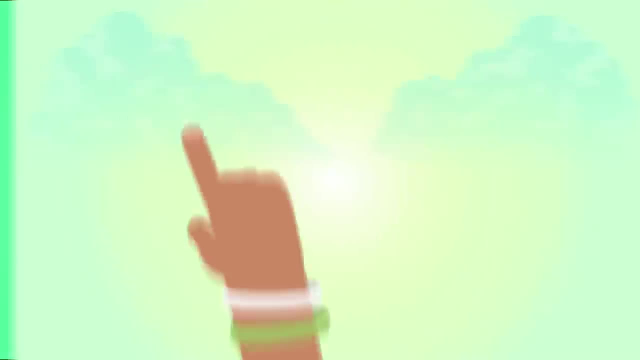 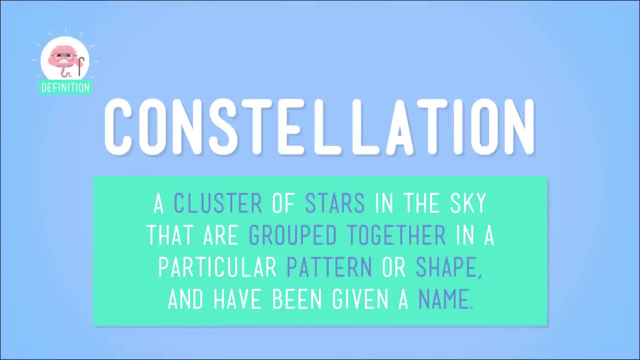 know what I mean. So what exactly is a constellation? A constellation is a cluster of stars in the sky that have been grouped together in a pattern or shape and have been given a name. But before we take a closer look at constellations, let's 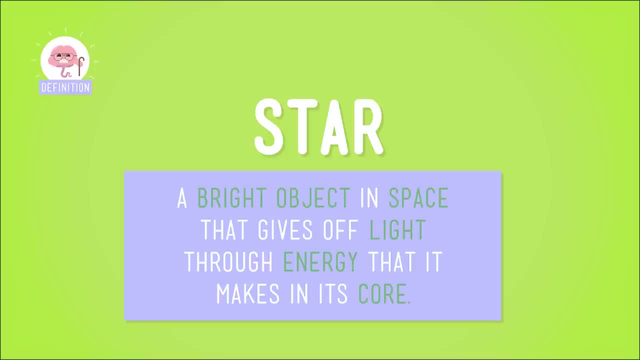 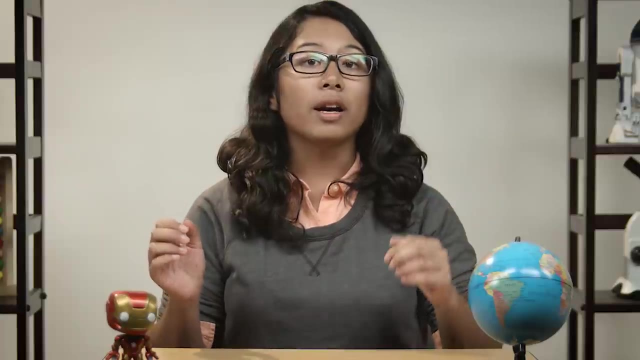 review what a star is. Remember, a star is a bright object in space that gives off light through energy that it makes in its core. The sun is the most famous star to us Earthlings. We've already talked about a few other well-known stars, though, like bright Betelgeuse Astronomers. 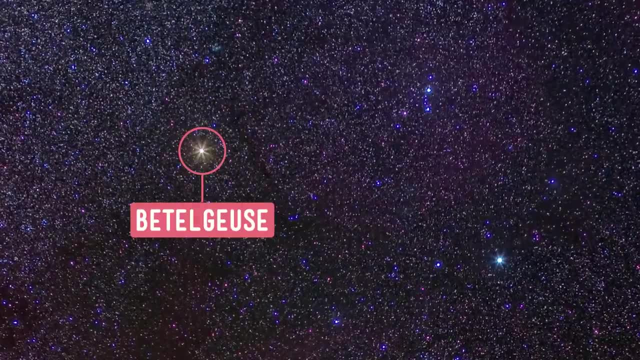 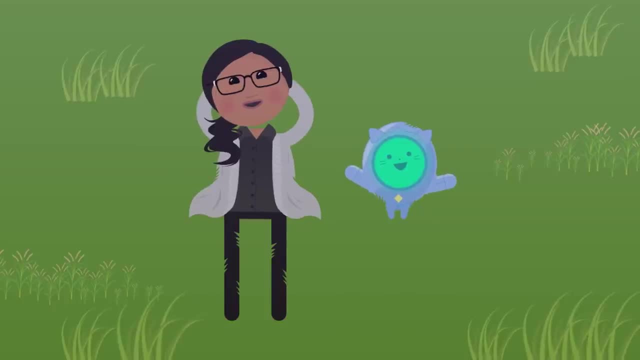 use bright stars like Betelgeuse as markers in the sky to help find other less bright objects in space. For example, if you were looking for a dim star like Sirius B, you might have to look for a long time to spot it among the many, many, many, many other stars in the sky. But 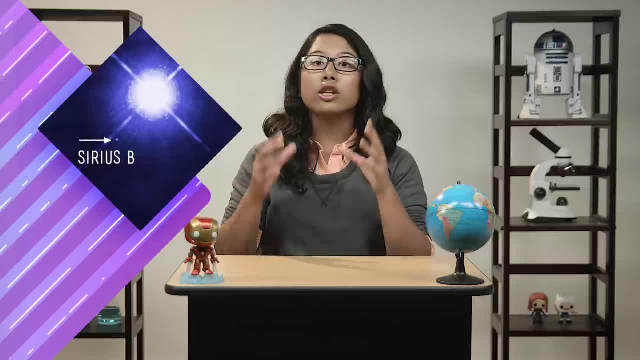 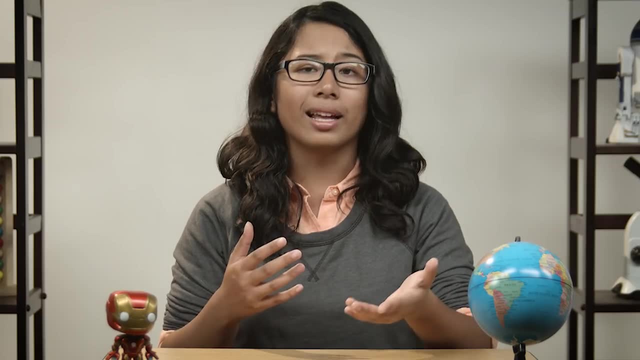 if you're able to spot a much brighter star like Sirius A and you know that Sirius B is located to the lower left of Sirius A, then it'll be much easier to find Sirius B. Like I said, there are so many stars in the sky that trying to spot just one can be. 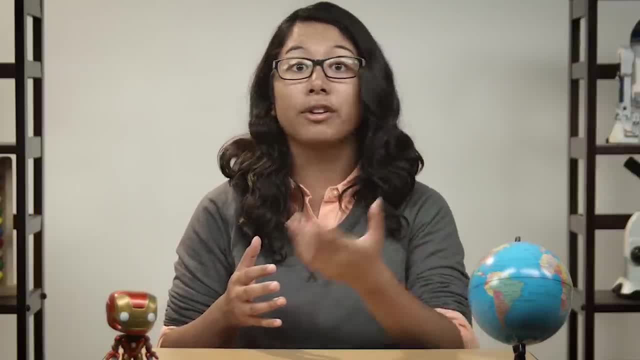 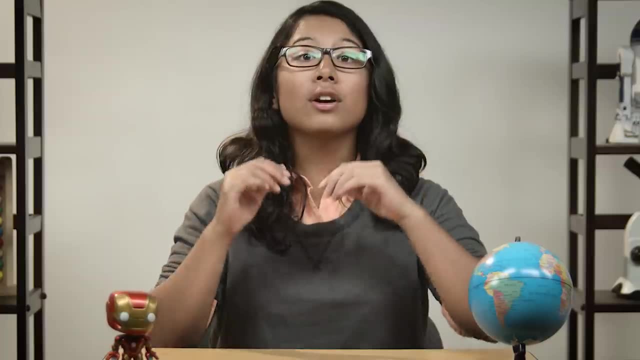 tough, Especially if it's not near a bright one like Betelgeuse. That's where constellations come in. Astronomers use constellations to help them better map the night sky. Think of stars like cities on a map and constellations like countries. 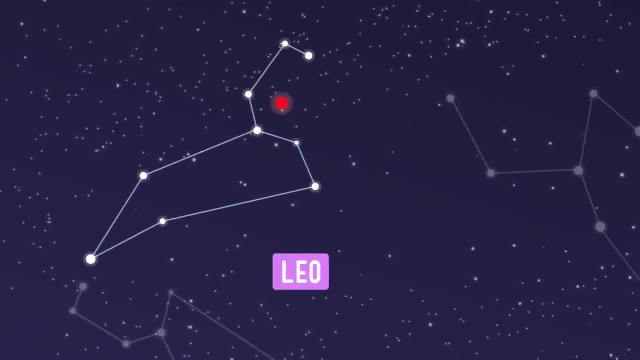 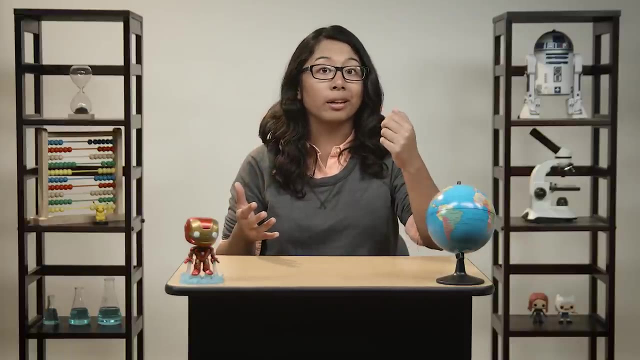 Finding a large shape in the sky made of many stars is a lot easier to spot than trying to find one single speck. Plus, there are only 88 named constellations, which is a much more reasonable number to deal with than a billion, And most of the 88 recognized constellations came from the 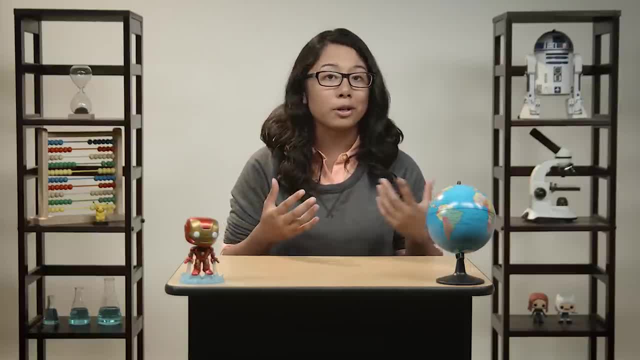 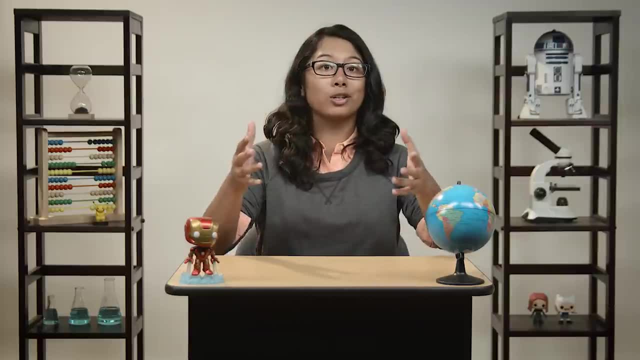 ancient Greeks, The stars in a constellation aren't related in any particular way. They form a shape that the Greeks used to tell stories about their gods, goddesses and mythical creatures like flying horses and giant scorpions. Now that we know what a constellation is, why don't we get to know some of the more? 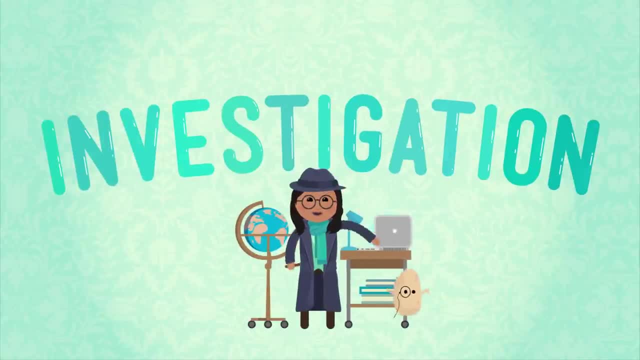 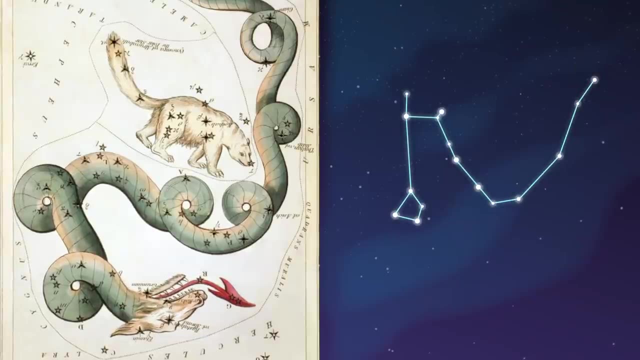 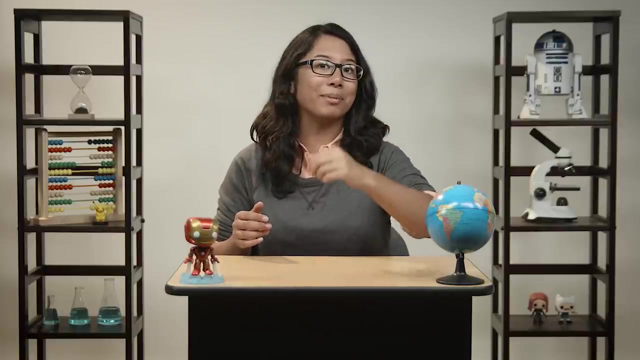 famous ones. Harry Potter fans will recognize the name of our first constellation. Its name means dragon in Latin and also happens to be the name of Harry's biggest nemesis- Well, second biggest, after Valthe, who must not be named, of course. 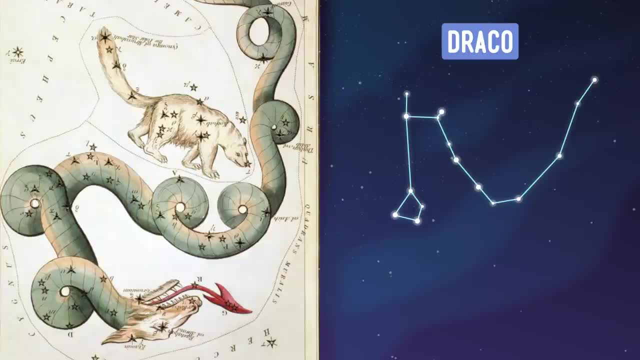 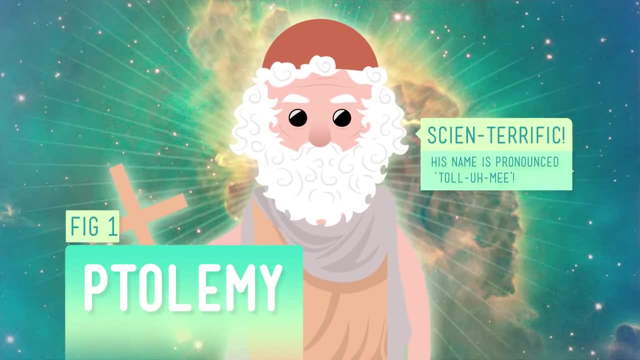 Yep, it's Draco. According to legend, Draco was a dragon killed by the goddess Minerva and was tossed into the sky. Draco is one of 48 constellations described way back in the second century by Egyptian astronomer Ptolemy. People have been seeing this dragon-like shape in the night. 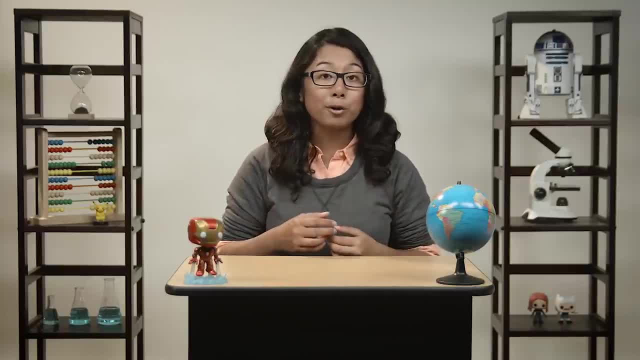 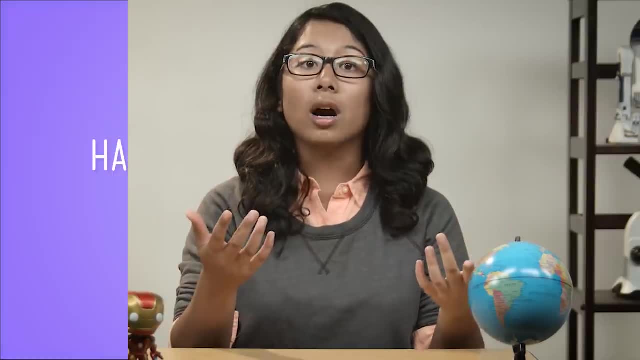 sky for a long time. Constellations aren't just named after creatures, though. Some are named after mythical people, particularly gods and goddesses. One of the more well-known Greek gods has his own constellation and a Disney movie. I'll give you a hint: He'll go there. 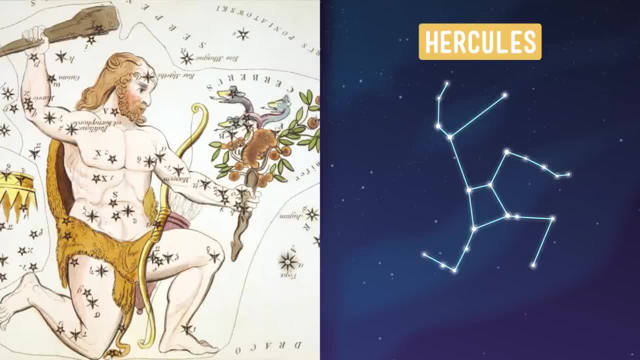 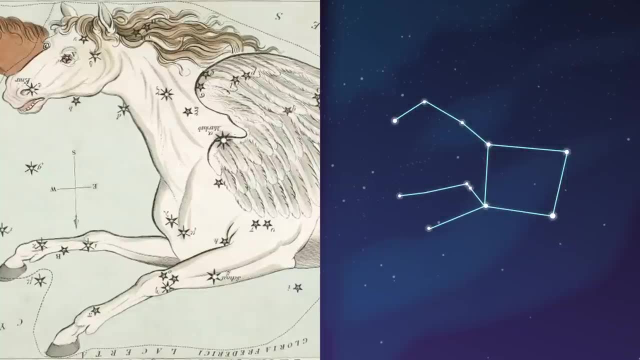 Follow the distance. It's Hercules. The stars in the Hercules constellation take the shape of the mighty hero, as if he's holding a bow. after just releasing an arrow, You go. Hercules, The name of our next notable constellation, also makes an appearance in the Hercules movie. 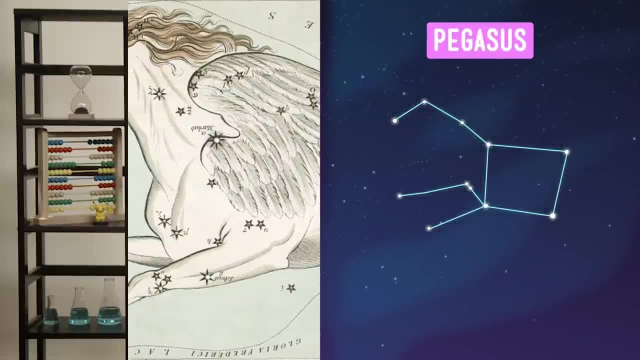 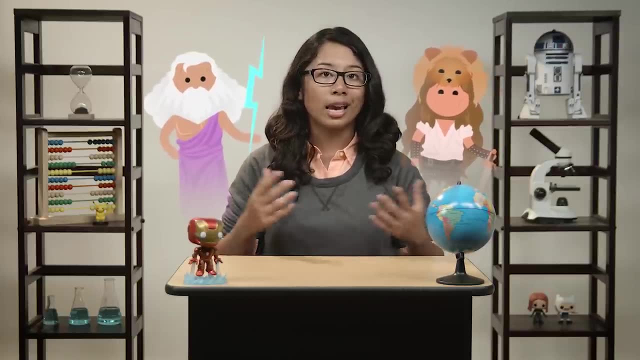 as a super cute winged horse, Say hello to Pegasus. According to Greek mythology, Hercules never actually rode Pegasus like in the movie, but the flying horse did spend some time with Zeus, king of the gods. Zeus liked Pegasus so much he transformed him into a constellation and placed him in 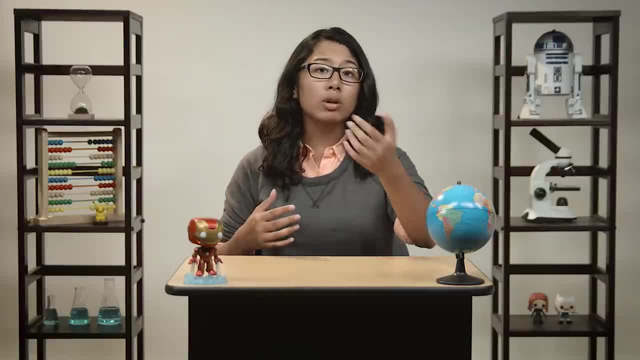 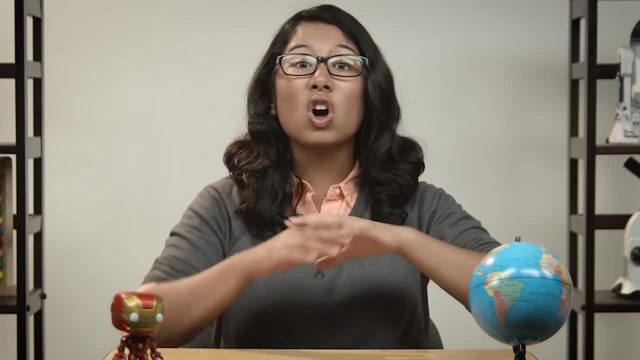 the night sky for every week. Now you're familiar with at least three of the 88 constellations in our sky. Only 85 more to go. As the Earth rotates. you'll see Draco, Hercules and Pegasus, plus all the other constellations.